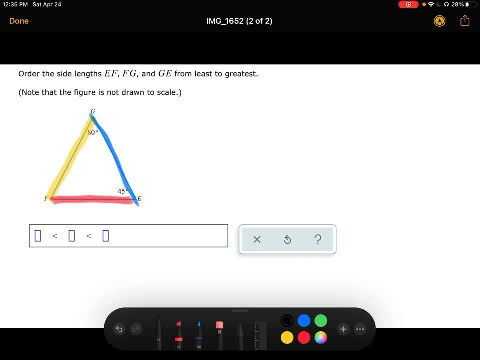 And I know you guys are like you can't figure that out. Ms Evans, I know You're going to learn it today. Okay, so this is sort of a two-step question. So the first thing you need to know how to do is you need to solve for this angle. 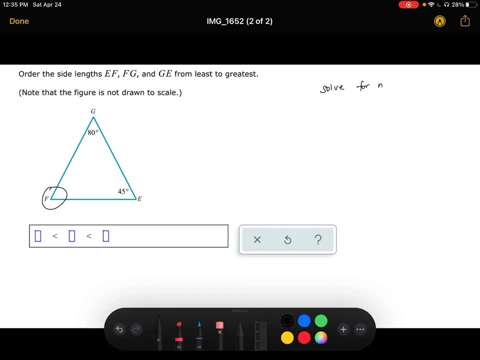 So solve for missing angle. you know, And I know someone's like, that has nothing to do with what we're talking about. blah, blah, blah. Somebody's already turned off the video and just asked me for help And I probably told you to come back. 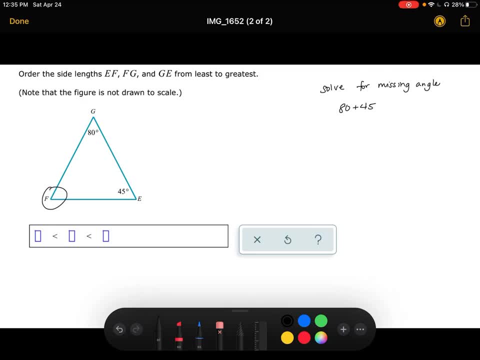 Come back and watch it again. You're fine. So the first thing you're going to do is you're going to add these two up right And that's 125, and then you're going to strap that from 180 to find the missing angle. 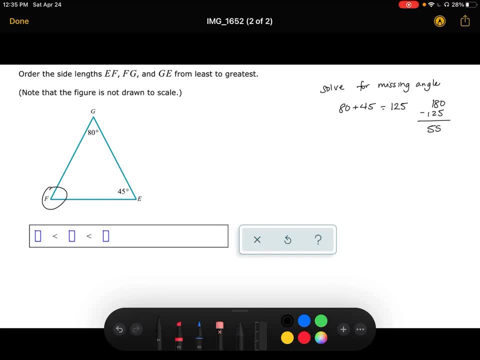 Put that in the calculator, because I tend to do these things wrong when I'm making videos. Okay, so the missing angle, so angle F, is 55 degrees. I know someone's like you're so slow doing math, Yeah, whatever. 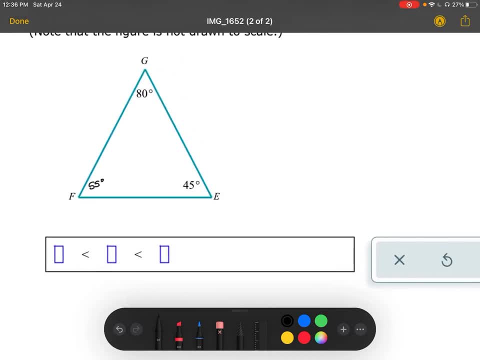 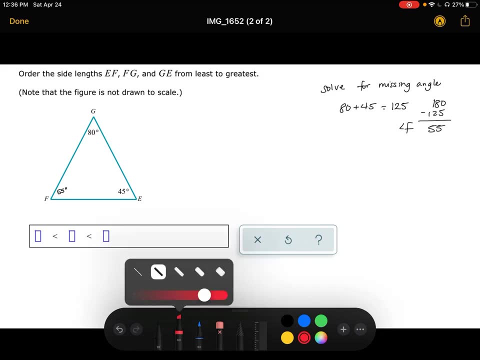 So here you go, 55 degrees. So this is the part that you now need to know, The angles, right. so let's say I'm going to put this in red. So angle F right here is right there. Now, when you look at this, this angle sort of points, not really, but it's opposite this side. 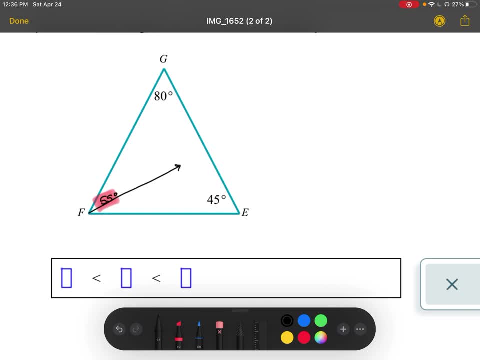 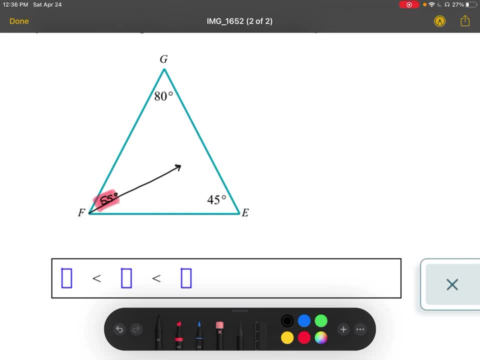 Okay, Okay, Okay, Okay, Okay, Okay, Okay Every time. Okay, that's just the way that it is. So I'm just going to put this out there, I'm going to highlight that out there, And this is GE segment GE. 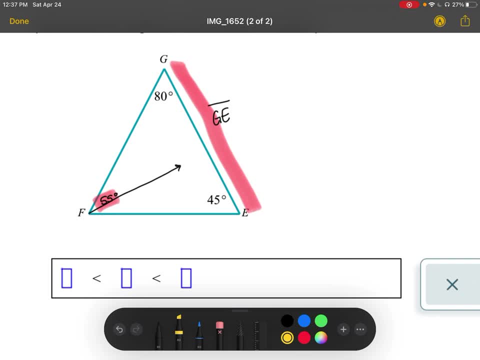 Okay, And then I'm going to do E, which is 45.. And that has a direct relation to- I'm just going to put this out there- and I'm going- That has a direct relation to E- to this one over here which is FG, an FG segment, FG, And let's do green. And then 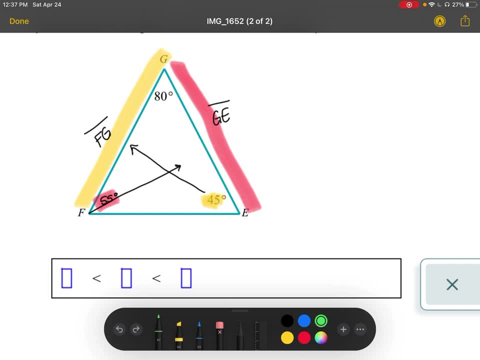 angle G, not the right one. Angle G has a direct relation to side FE. Okay now, these direct relations are essentially saying that the angle relates to the side length. So angle angle G right is the same as FE, segment FE. Well, they have that relation And this is. 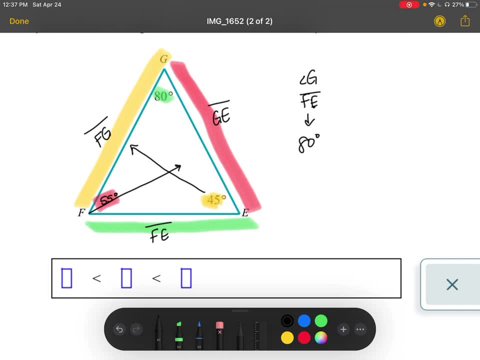 80 degrees. Okay, that is the longest one. So, because they're in relation to each other, angle G is the biggest angle, so angle F is the longest side. Okay, that's just the way that works And I know this. 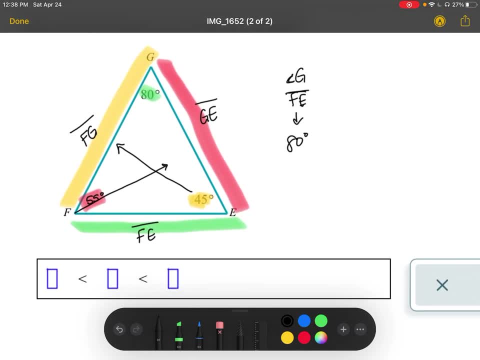 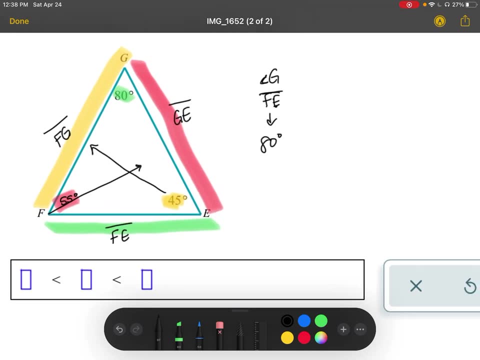 looks like an equilateral triangle, But it tells you the figure is not drawn to scale. they do that because then you would just say it's that one and you wouldn't have to actually do the math or understand the reasoning. Whatever, we like to trick you guys, Anyway. so the next one I would 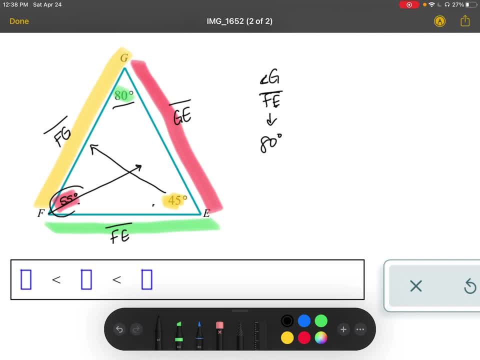 say okay, well, there's 80.. The next one: I have two levels: 55 and 45.. Well, 55 is the next one. So I know that's angle F And that corresponds to GE, And that is 55 degrees. And then the last one is angle E. 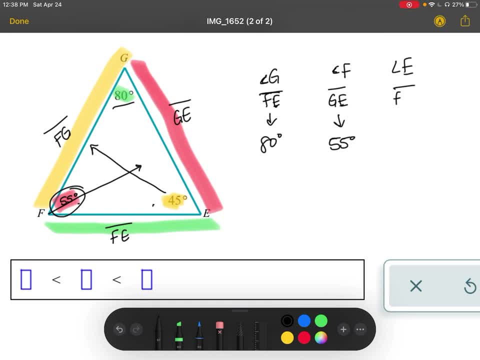 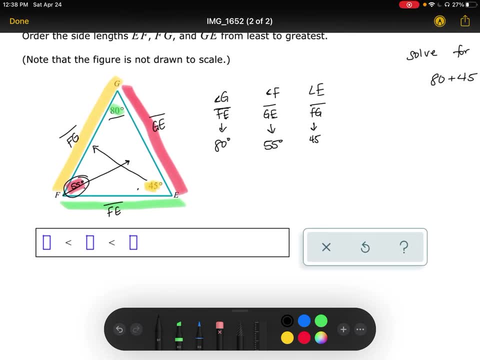 which angle E, which corresponds to mine, FG, which is 45 degrees. So I know I wrote this backwards, but it's least the greatest And my bad should have wrote that backwards. But there we go, I can just put that in there. So I know that the smallest is segment FG, So I'm going. 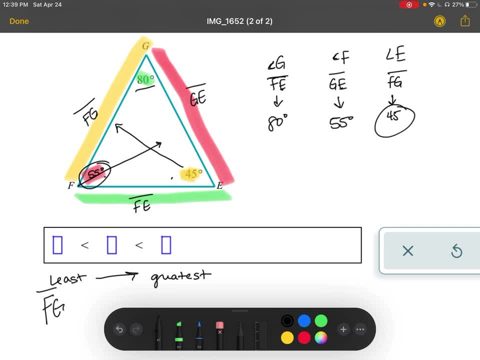 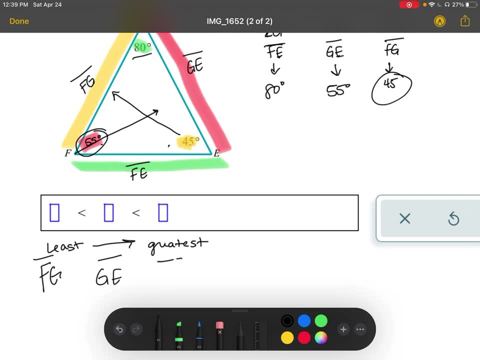 to say: I'm just writing down here FG, And then the next one is GE And the next one is FE. All right, guys, that's all you need to know. It's a really simple concept, And I know that. I took the. 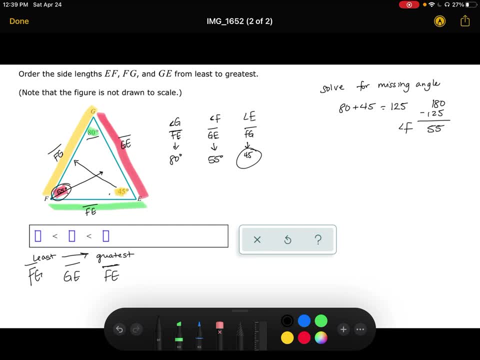 longest route. some of you guys are visual learners and you call it an explanation And there you go. So if you need another explanation, or you're just confused, or whatever it is, just go ahead and type it in the comments And I'll see you guys in the next one. Bye.